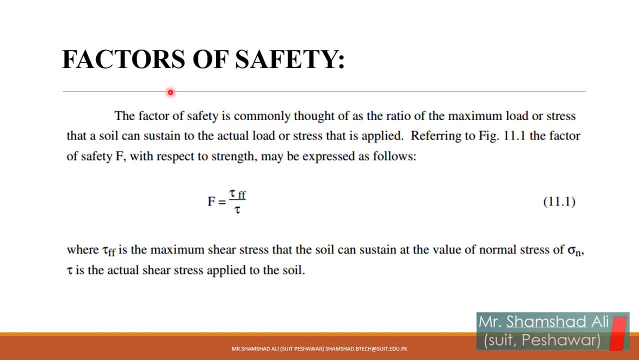 design and other engineering structure is somewhat different from the factor of safety of the stability of the slopes. The factor of safety is commonly thought of as the ratio of the maximum load or stresses that a soil can sustain to the actual load and the actual load of the material. 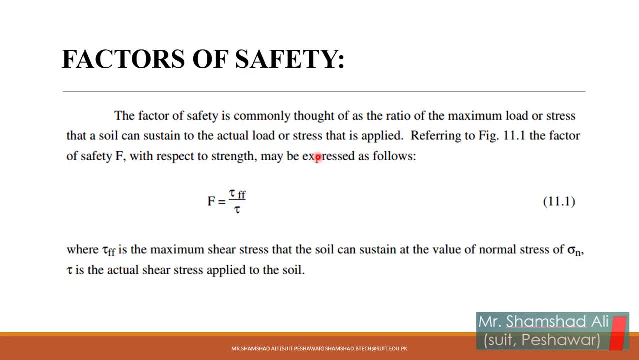 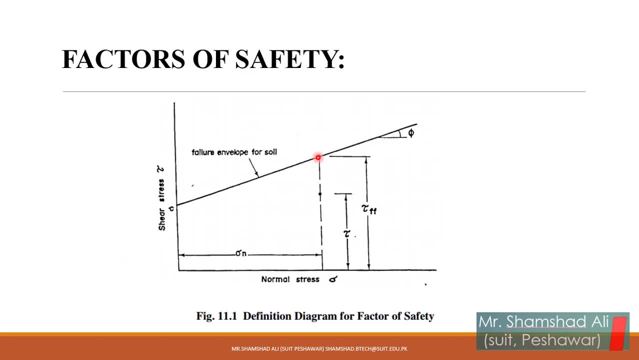 a stress that is applied. referring to figure number eleven, point one one, this is basically difficult. 11.11 definition diagram for factor of safety. here we have the normal stress, here we have the shear stress. this is the cohesion, this is the failure envelope of side. just like this, this diagram is being developed. 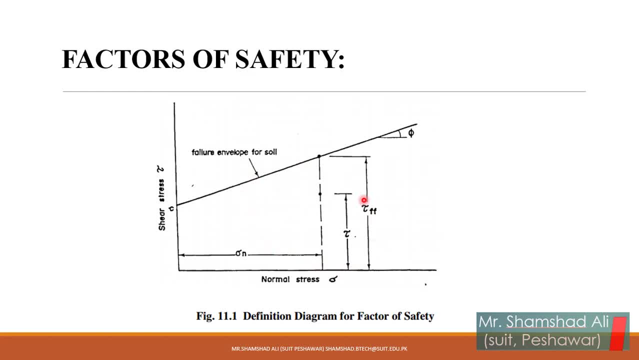 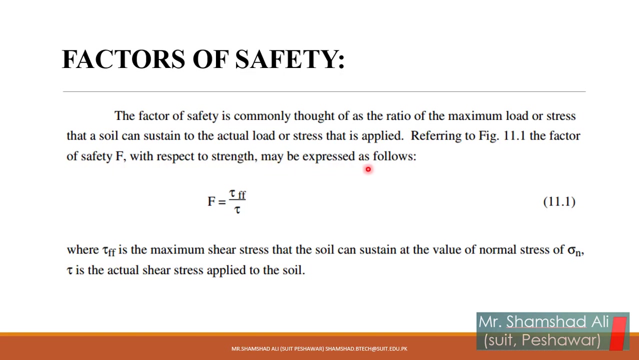 from the Mohr-Coulomb failure envelope. this is the angle of internal friction. this is basically the tau FF and the tau, this is the normal stress. so the figure, the factor of safety F, with respect to string may be expressed as follows: here we have: the F is equal to tau into FF divided by the tau. 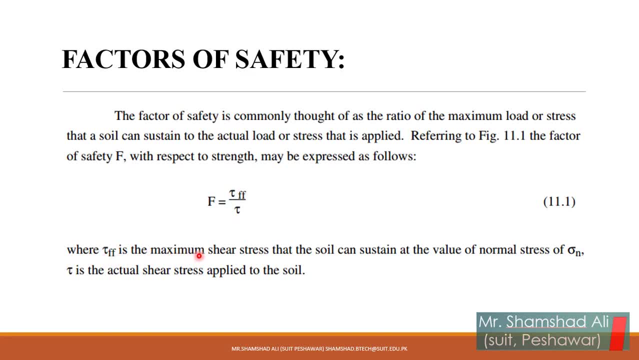 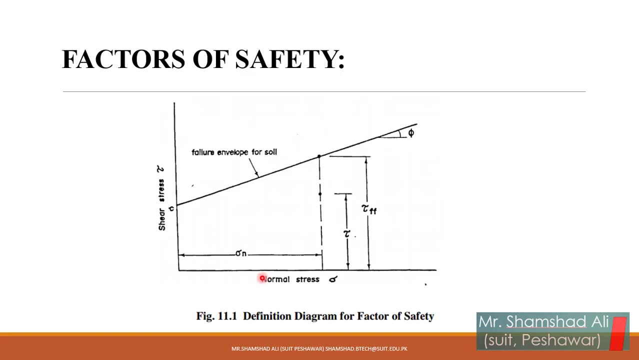 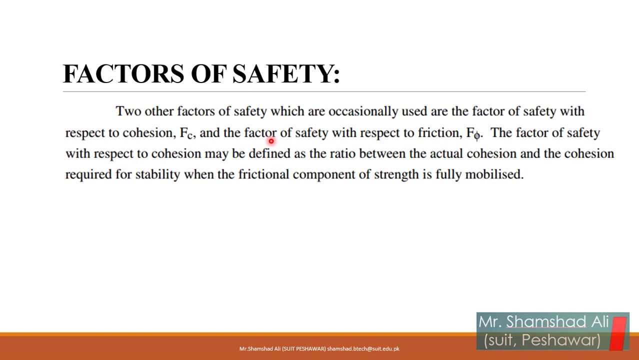 where T, tau into FF, is the maximum shear stress that the soil can sustain at the value of normal stress, of normal stress, of the minimum, then tau is the actual shear stress applied to the soil. this is basically the factor of safety. two other factor of safety which are occasionally used are the factor of safety with 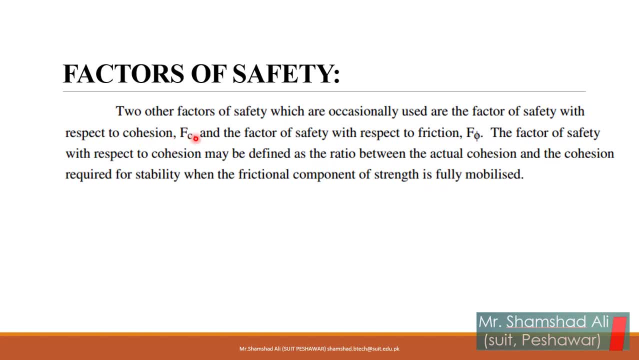 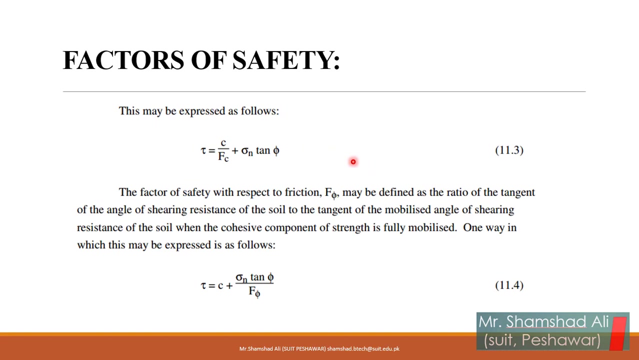 respect to cohesion and the factor of safety with respect to fraction. the factor of safety with respect to cohesion may be defined as the ratio between the actual cohesion and the cohesion required for stability when the fractional component of string is fully mobilized. this may be expressed as follows: tau is equal to C divided by the. 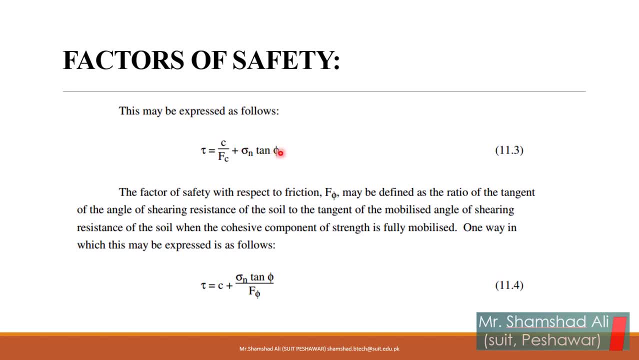 F, C plus normal stress tangent into theta. the factor of safety with respect to friction may be defined as the ratio of the tangent of the angle of shearing resistance of the soil to a tangent of the mobilising the left shearing resistance of the first mình, the cohesive 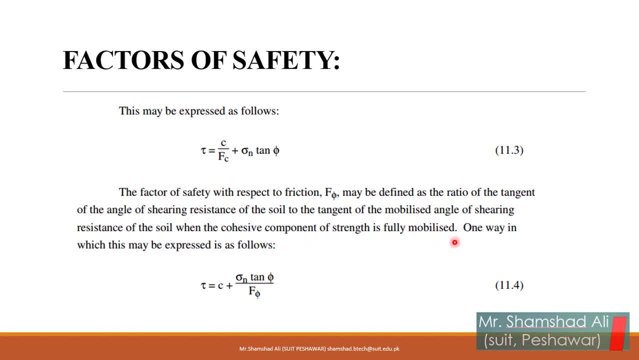 component of the strength is fudui liking day. one way in which this maybe space is esparno, as you could a st e karena sasenho target. he's already played 50, think it. this is the dispute. effector of safety for the cohesion, for the fraction. 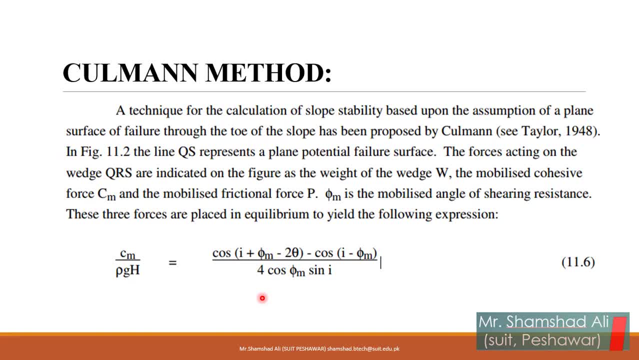 colman method. now we are going to only discuss- remember that we are going to discuss- just the methods which are used for the analysis of the slope stability. a technique for the calculation of the slope stability based upon the assumption of a plane surface of failure through the toe of the slope has been proposed by colman c taylor 1948 in figure 11.2. 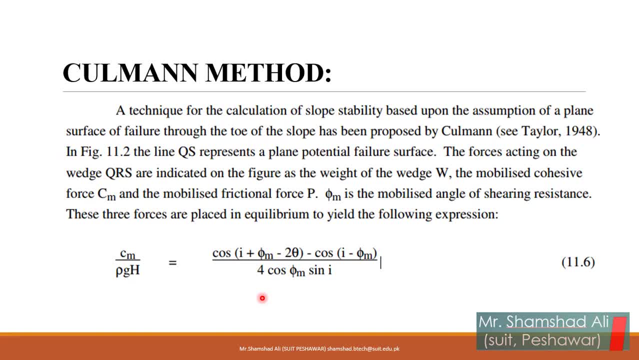 the line q is represent a plane potential failure surface: okay, surface. the force acting on the wedge, qrs, are indicated on the figure as the wave of the bridge. w, the mobilized cohesive forces, cm and the mobilized fractional force, p into t. time to n is the mobilized angle of sharing resistance. these three forces are: 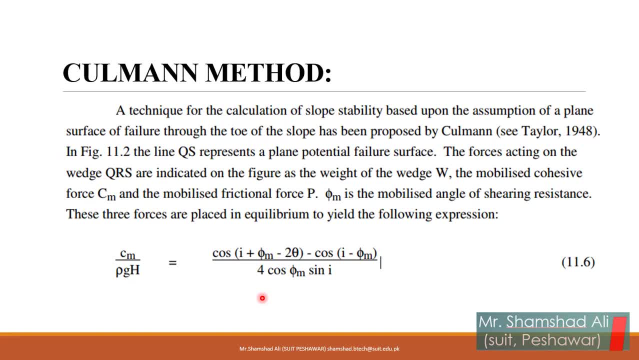 placed in equilibrium to yield the folding expression. basically, the colman method is the method of the equilibrium when these three terms are in equilibrium. so we can express the mathematical form of the analysis that the ac into n mean. the mobilized cohesive force divided by p into g, into h, is equal to cos of the i plus. 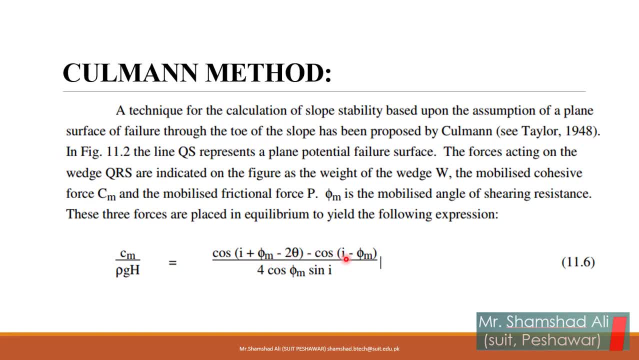 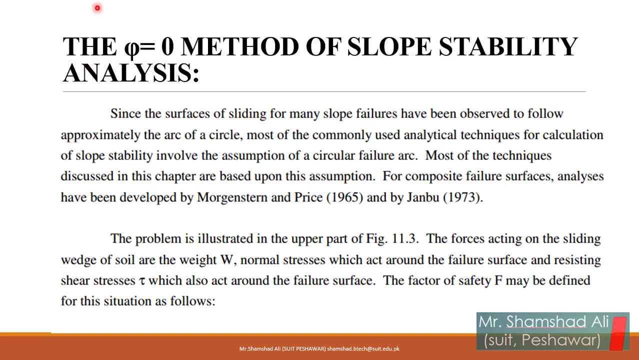 theta into m minus 2. theta minus cos i minus theta m divided by 4 into cos. theta m into sine i. okay, the theta is equal to the angle of internal fraction 0. method of the slope stability analysis. this method is used for the style or the cohesive style. basically, since the surface of sliding, for many slope failures have been. 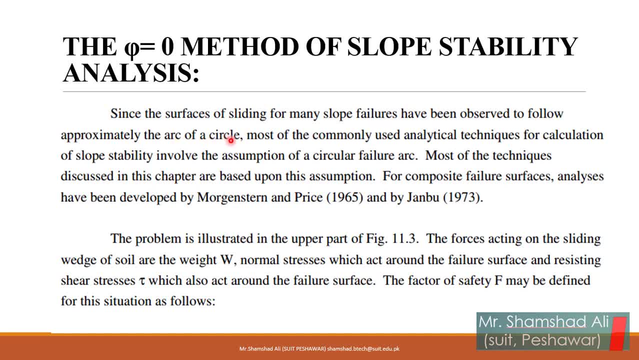 observed to follow approximately the arc of the circle. most of the common used analytical techniques for calculation of slope stability involve the assumption of a circular failure arc. most of the techniques discussed in this chapter are based upon this assumption. for composite failure surfaces, analysis have been developed by morgeson and price in 1960s. 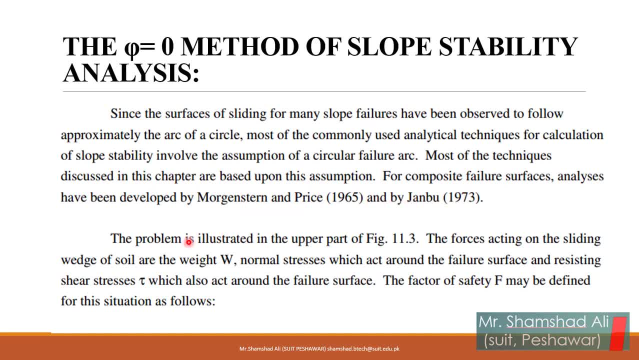 and by john boo in 1973.. the problem is the study in the upper part of the figure 11.3. the force is acting on the sliding wedge of of soil. uh the wave w normal stresses a which in on the failure surface and resistance share. uh resisting shear says star which also act around. 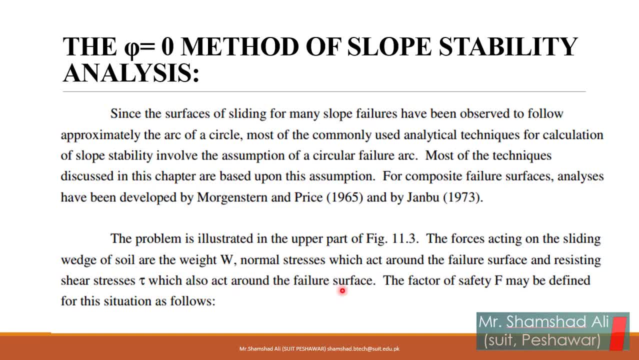 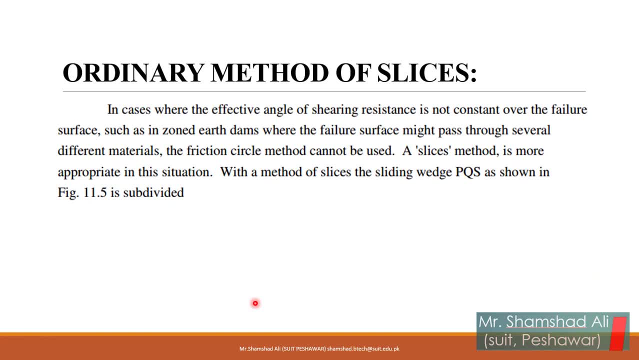 the failure surface, the factor of safety may be defined for this situation is followed. the field is is represented by these three as 연� prix by ord 19 methods of slices most commonly used. method an is the ordinary method of the slicing other than also we use, but in literature as i have learned that the slice method is used most founding in cases where the effective angle of shearing resistance is not constant over the Change, the unknown surface, such as in zones of dams where the你的 surface end Nikáis concealer subsolie. often it turned kind of crack at that point such that it means that ketchup lead surface and the strength of the surface surface, such as in zones of dampness where the 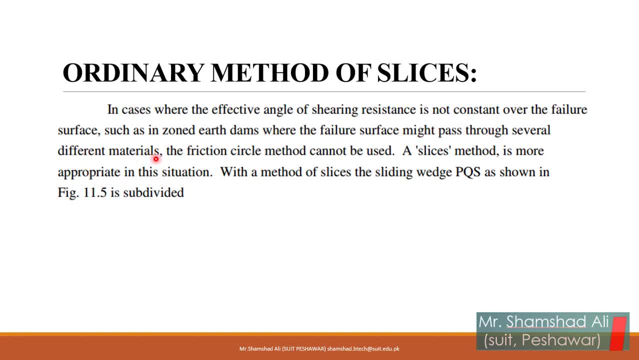 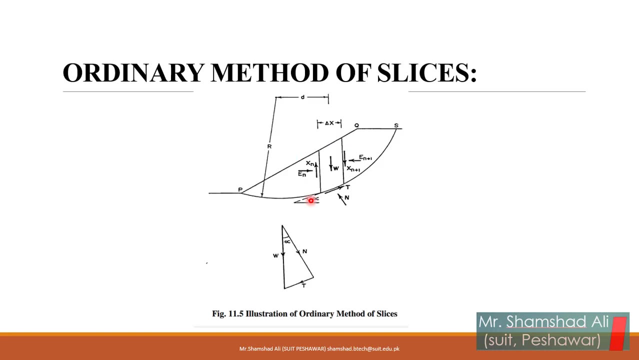 surface might pass through several different material. the fraction circle method cannot be used. a slice method is more appropriate in this situation where the method of slices, the sliding, which pqs is shown in the figure learn the fire is subdivided. as you can see, this is basically the slice first mean a. 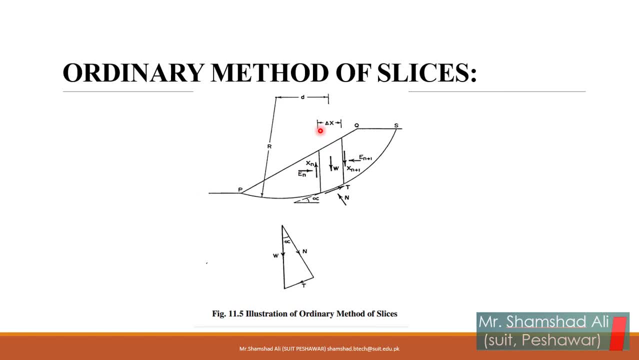 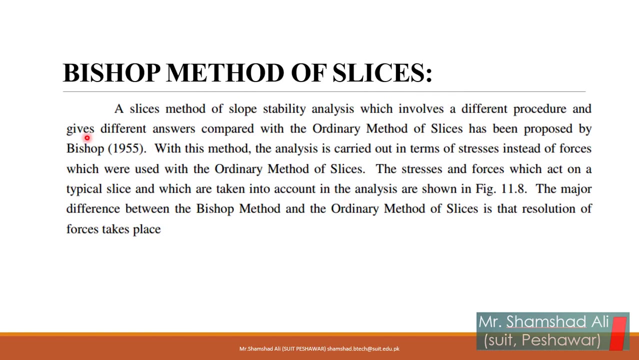 piece which will be analyzed. this is the delton to a was a W. this is the X into n. this is the end to end, and this also this year, and illustration of ordinary method of the slice bishop method of strikes the slide, a slice method of slope-severed analysis, which involve different procedure and give different 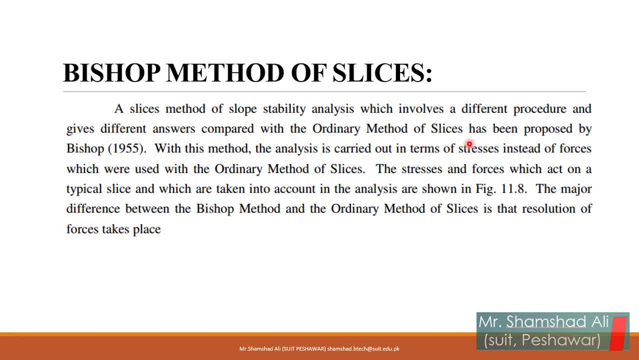 answer: compared with the ordinary method of slices, has been proposed by Bishop in 1950, where this method, they knowledge, is carried out in terms of stresses and still forces. victory were used with the ordinary method of slice, the stresses and forces with it on the typical slice. 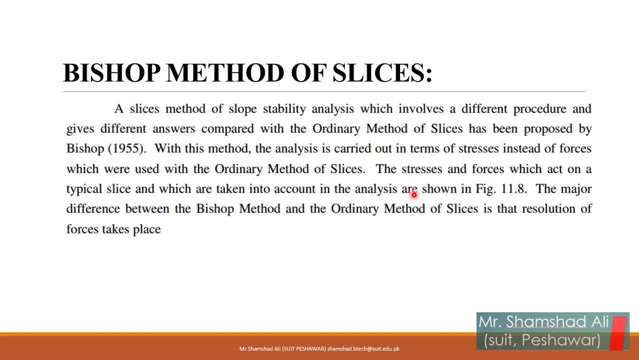 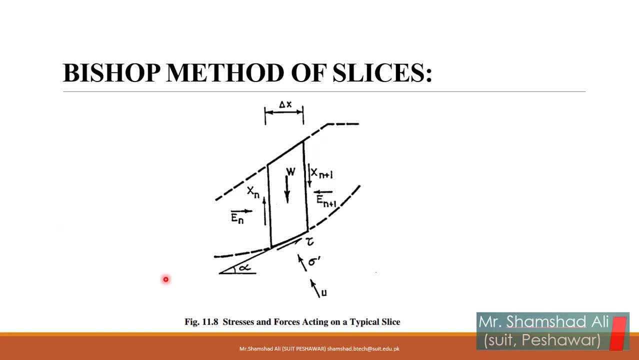 and which are taken into account and the analysis are shown in figure 11.8. the major difference between the bishop method in the ordinary method of slices is their resolution of forces take place- this- this is basically the bishop method of the slices- short-term and long term stability. this 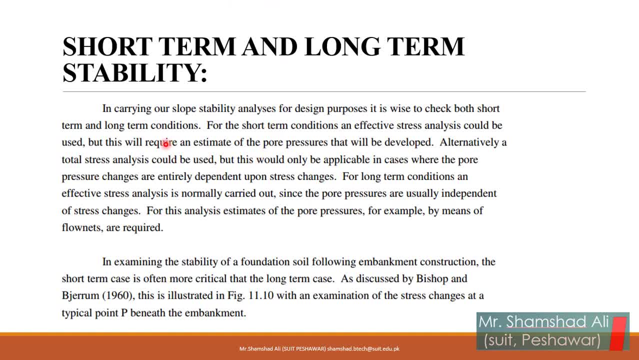 is the most important part of today's picture in kingdom, or slow stability analysis by design purposes. it is wise to check both shortened in downtown condition when you are going to analyze the stability slopes, so you probably when you must have to check it for the shagger. 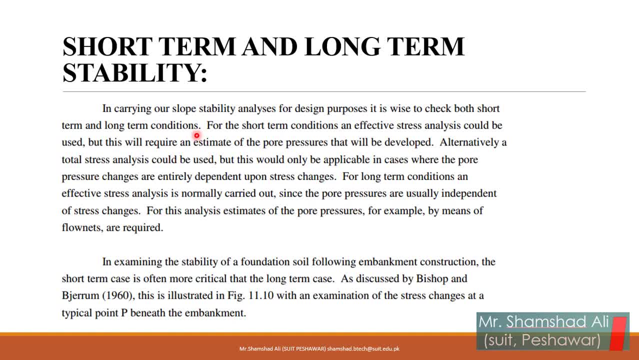 as well as for the long-term condition as well. for the short-term condition and effective stress analysis could be used, but this will require an estimate of the pore pressure that will be developed. these are the main point that for the short-term condition, effective stress analysis- the pore water pressure will be a- will be estimated. alternatively, a total stress analysis. 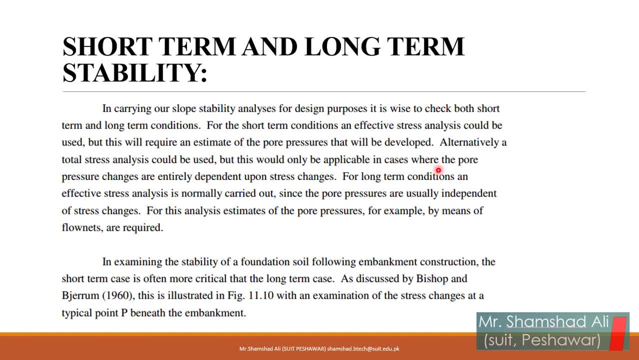 could be used, but this will only be applicable in cases where their pore pressure changes are entirely dependent on the stretch for long-term condition and effective stress analysis is normally carried out, since the pore pressure are used independent of stress chain. for this analysis, estimates of the pore pressure, for example by means of the flow nets, are required. 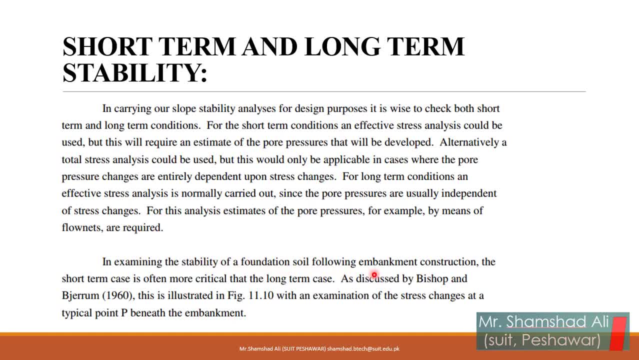 and examining this stability of a foundation side for following embankments construction. the short-term case is often more critical than the long-term case, as discussed by bishop and brim 1960. this is illustrated in figure 11 by 1: 0 with an examination of the stress change at: 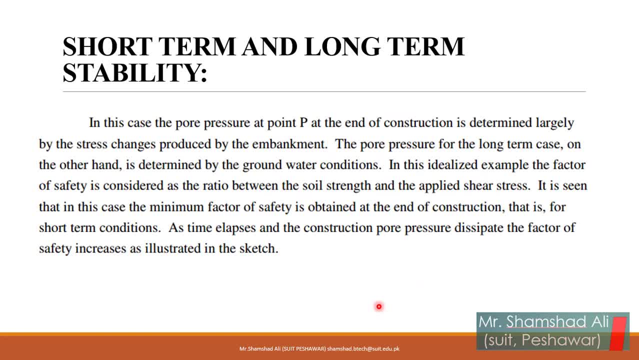 a typical point p beneath the embedments, in this case the pore percivite. point p at the end of the construction is determined largely by the stress chain produced by the embankment. the pore pressure for a long-term case, on the other hand, as determined by ground water condition in this idealized 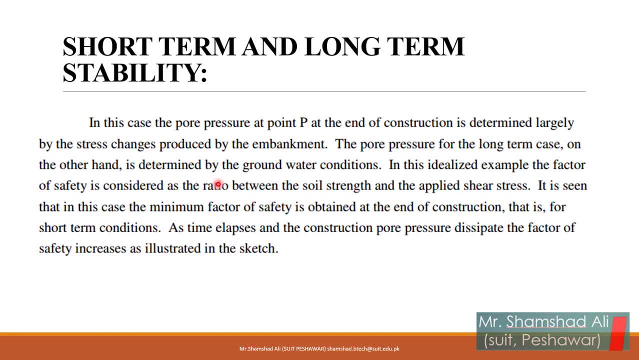 example, the factor of safety is considered as the ratio between the soil chain and the applied shear stress. it is seen that in this case, the minimum factor of safety is obtained at the end of construction, that is, for short term. condition is time elapses and the construction pore pressure dissipate. 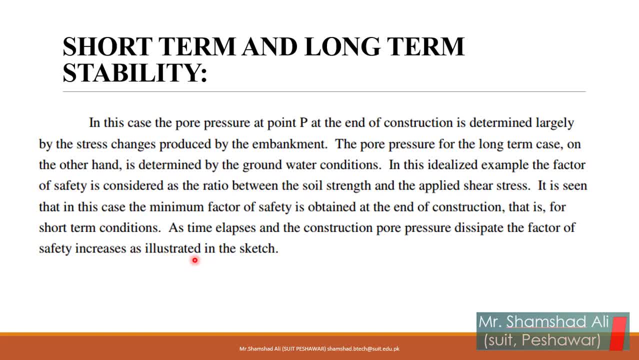 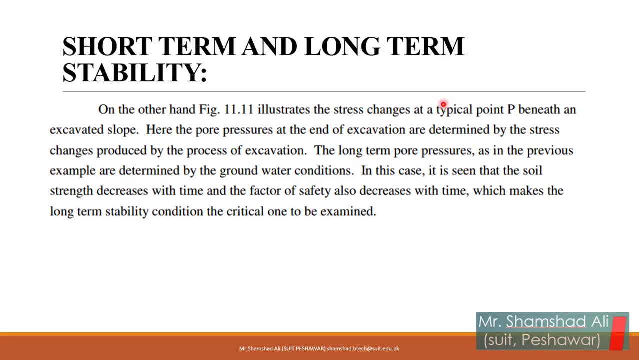 the factor of safety increase is illustrated in the sketch. on the other hand, a length, 1 moment- is set. this stress changes that the typical point P beneath an excavated stone. here the pore pressure at the in excruciation are determined by the stress chain to be by the process of accumulation. the long 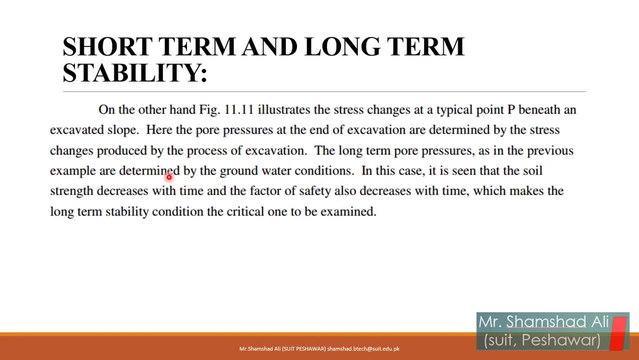 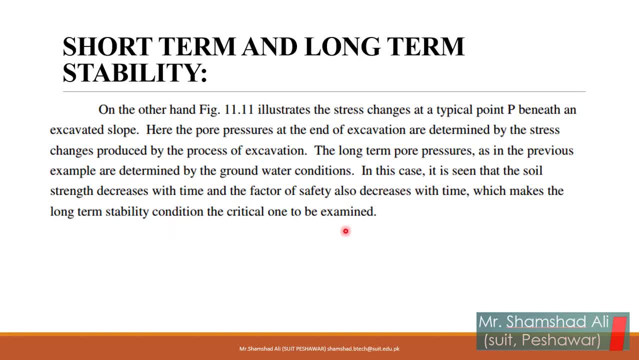 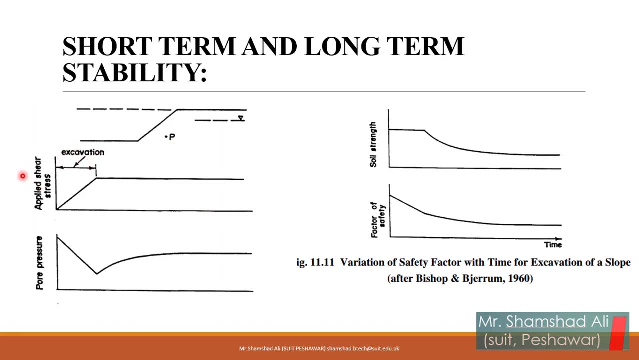 soil strength decreases with time and the factor of safety also decreases with time, which makes the long term stability condition the critical one. to be exact, This is the figure. this is basically the P. this is the excavation applied shear stresses. this is applied shear stresses pore pressure and the pore pressure increases soil strength. 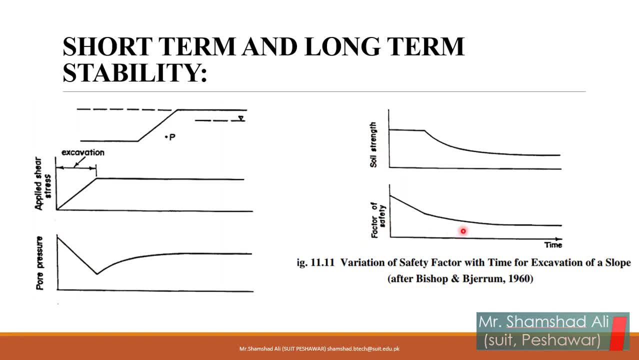 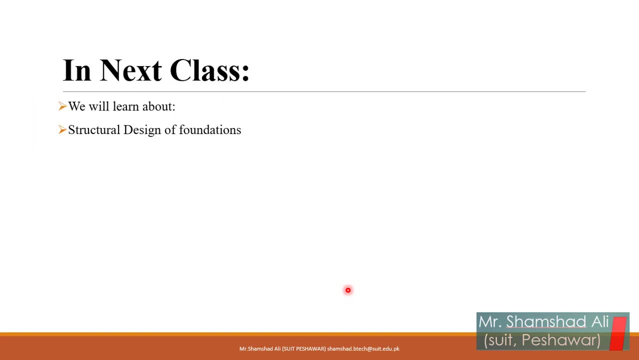 increase found in the factor of safety. Variation of factor of safety. safety factor is the time for excavation of a slope for Bishop and Byrne in 1960.. So this is it for today's class. Hope you will learn something about the methods which has used by the analysis of the slope stability. 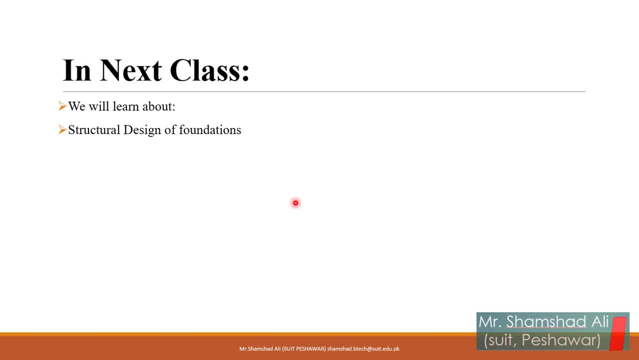 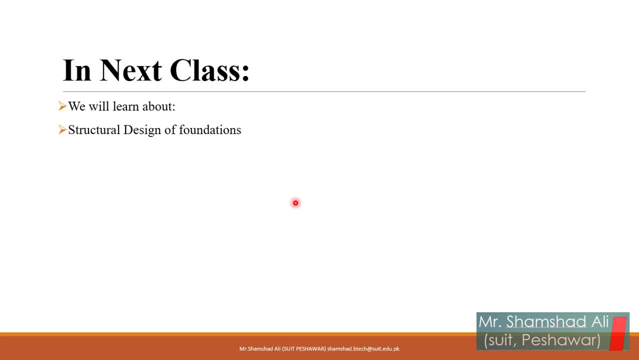 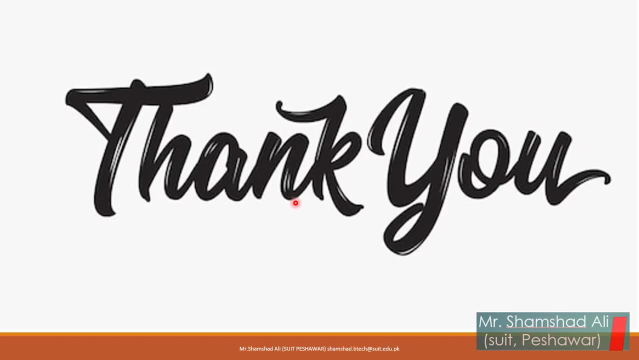